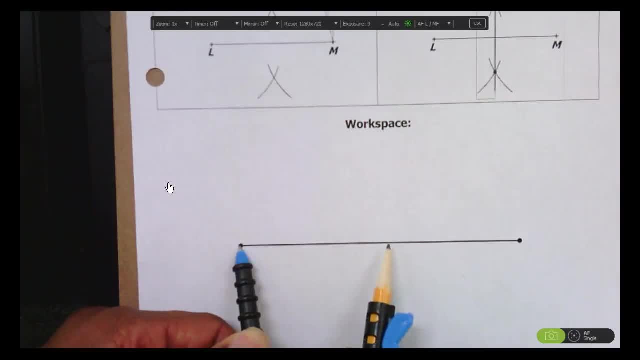 Now you need to open your compass more than halfway- All right. it has to go past the midpoint of the segment. It doesn't have to be exactly anywhere, but it needs to be more than halfway- All right. now go ahead and draw. 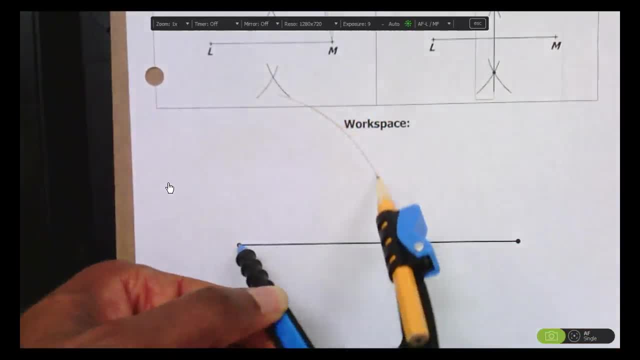 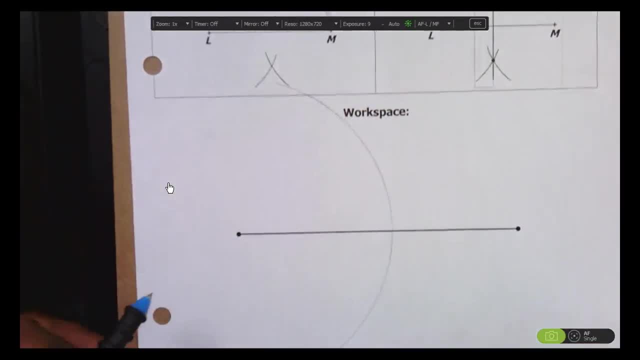 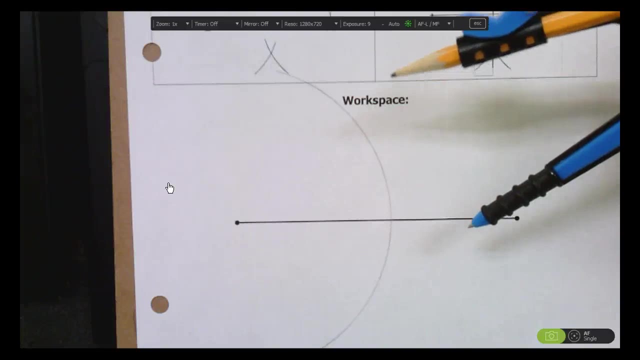 Draw yourself a big arc like this And then we're just going to switch sides. Don't change the size of your compass, Just leave the size of your compass exactly the same. Just move the point of your compass to the other end point. 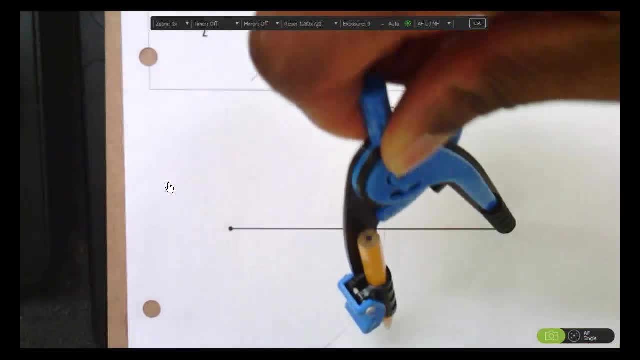 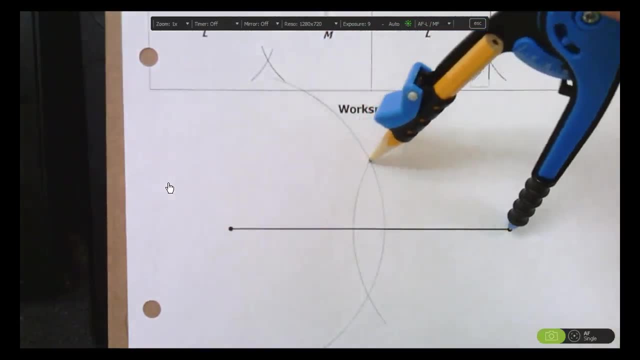 And then go ahead and draw an arc that will intersect Your The first arc in two places, like this. So guess what? Those two intersection points that you can see show you where the perpendicular bisector is going to go. Now I just lost my ruler. 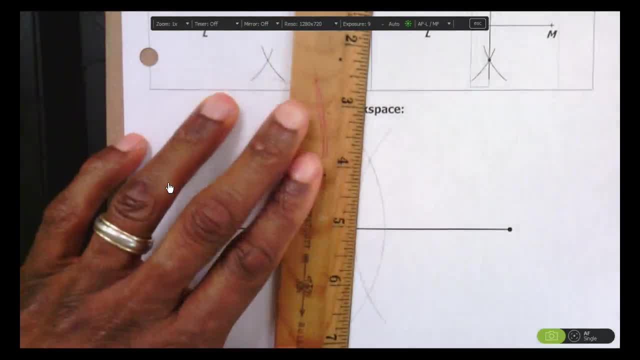 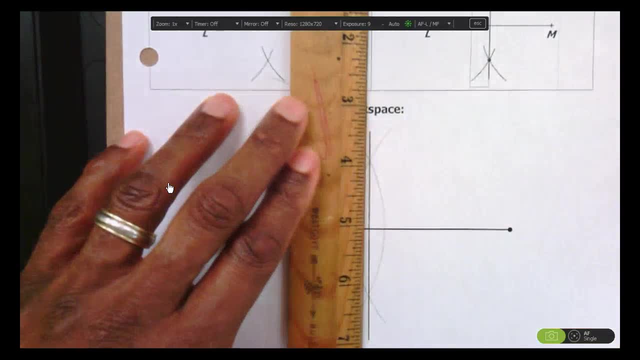 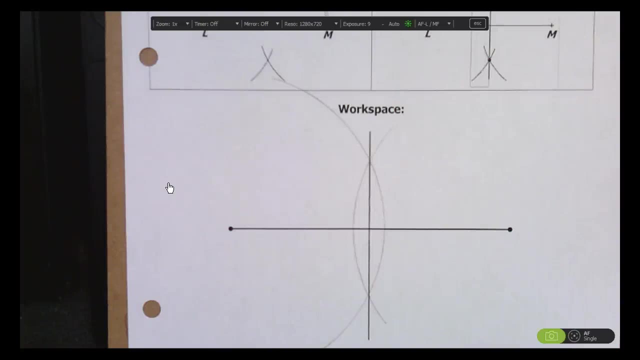 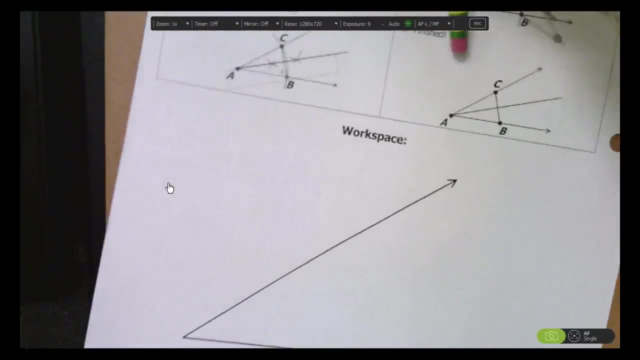 Thanks. Okay, so all you have to do is draw the perpendicular bisector Through those intersection points like that and boom, perpendicular bisector. All right, so now I'm going to show you how to construct the angle bisector. So flip your paper over and I'll show you how to do an angle bisector. 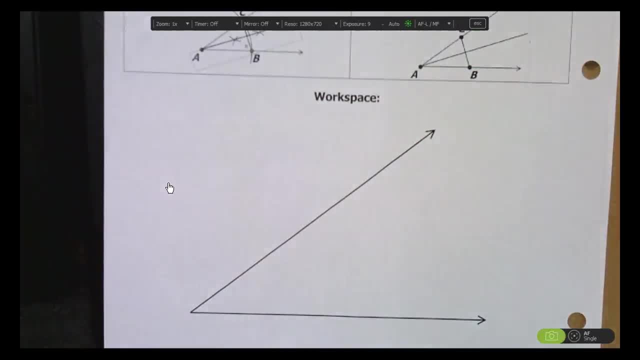 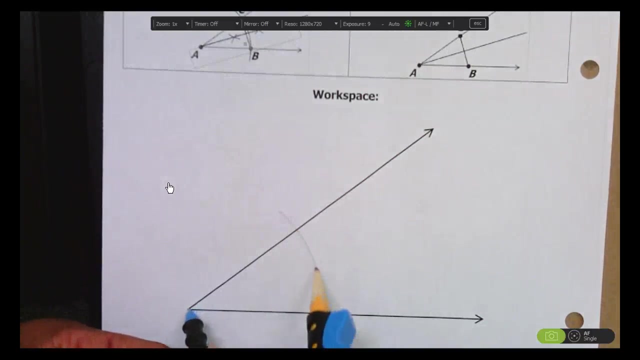 So take your compass, put the point of your compass at the vertex of your angle Now. it doesn't matter exactly how big your compass is right now, but draw yourself an arc that intersects both sides of the angle, like that. So, 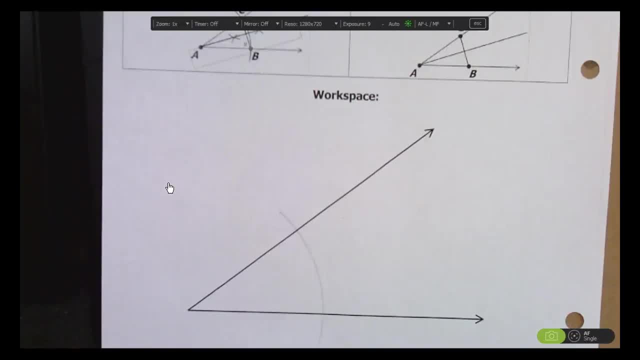 I just taught you how to do a perpendicular bisector of a segment, So all I'm really going to do now is I'm going to do the perpendicular bisector of this segment. See these two end points right here. All right, the two intersection points.